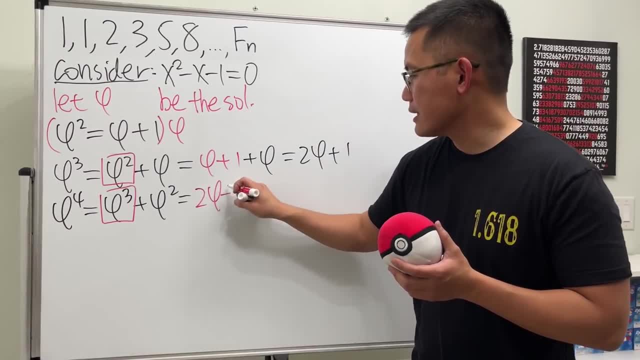 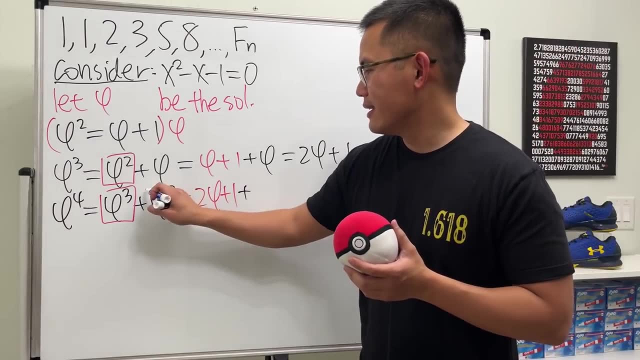 So I can just go ahead and say we will have 2v plus 1.. And then we just have to add phi squared, And I think we know phi squared is huh. This right here is just that, which is just phi plus 1.. 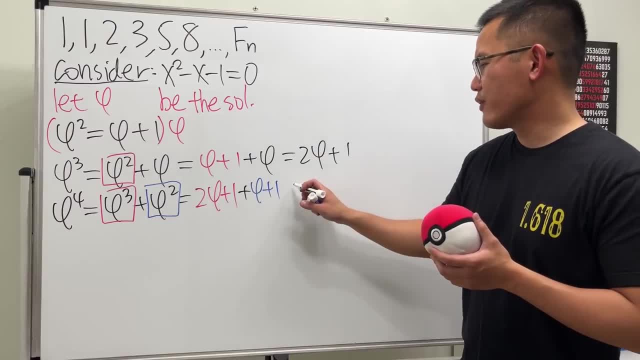 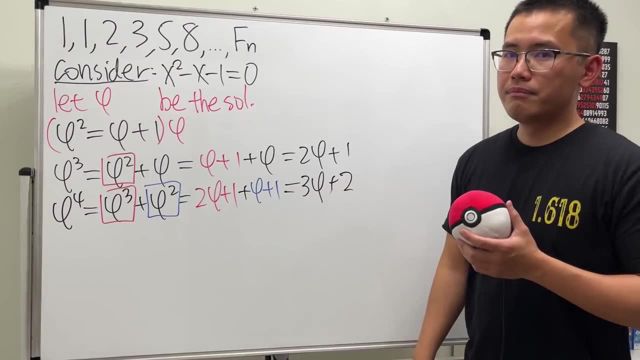 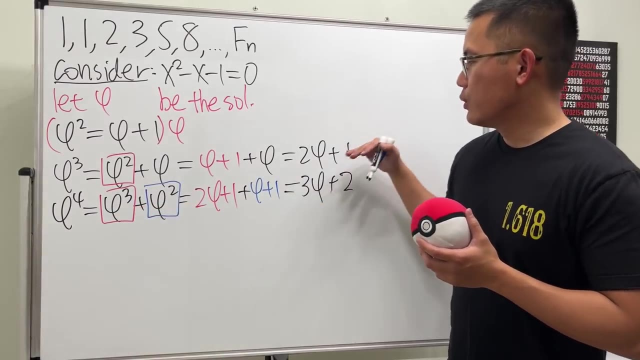 And can we just? Can we just go ahead and add them up? Yeah, of course It's 3v plus 2.. Good, But did you guys notice what we just did, phi to the third power plus phi squared, which is this plus that. 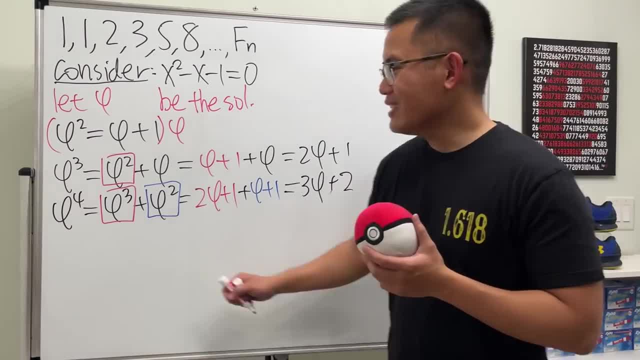 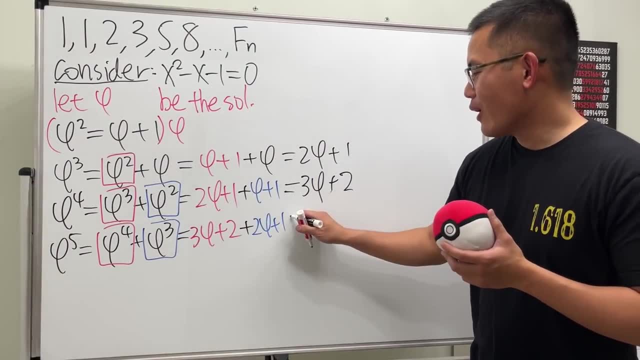 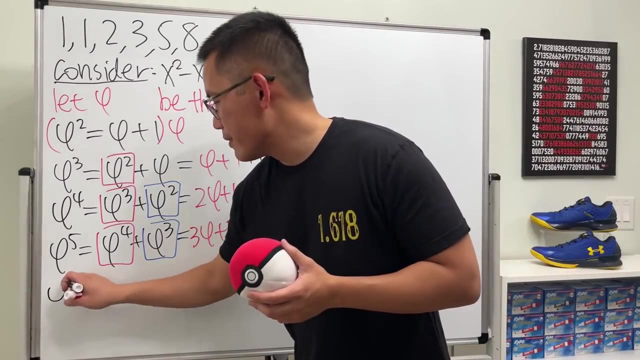 Okay, Keep that in mind. Let's do it again. Guess what? All in all, we get 5v squared, 5v plus 3.. Good, All right, Let's do it one more time. phi to the sixth power. 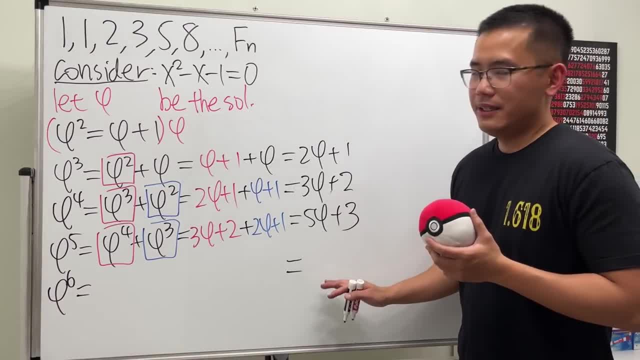 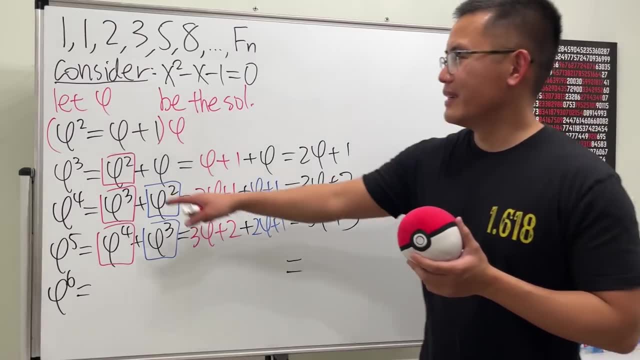 But this time I'm not going to write down the work, Let's just look at the pattern, if we can figure this out. Do you guys see the pattern? Yes, Look 1. And technically we can also backtrack here. 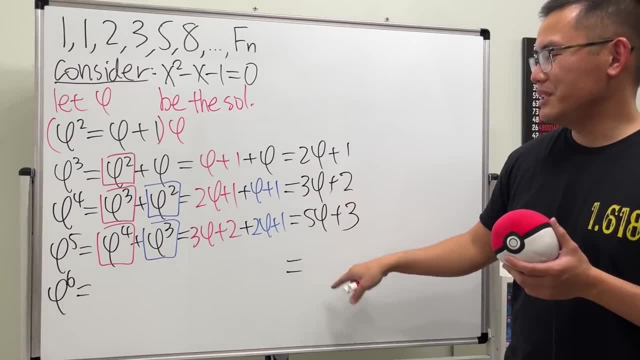 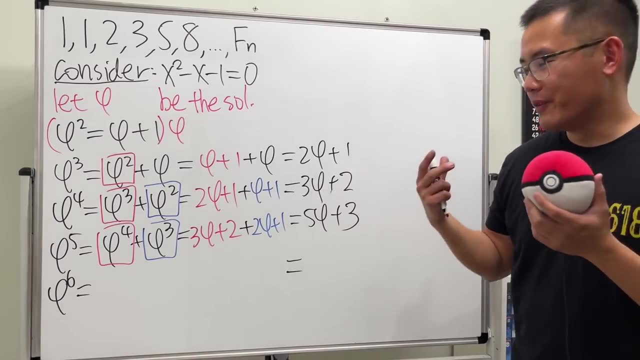 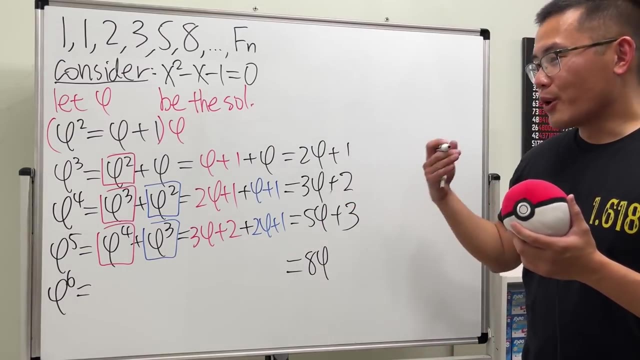 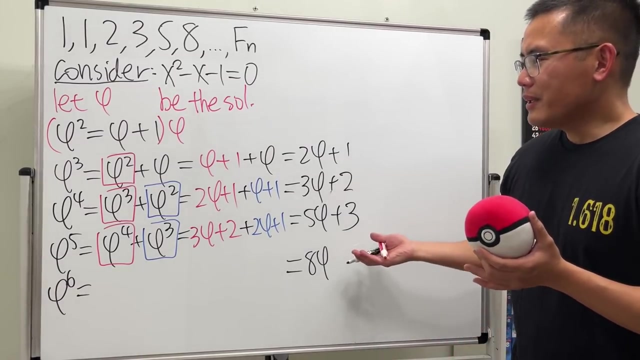 It's 1, 1,, 2,, 3, 5.. So what's the next one? 8.. Yes, They are the Fibonacci sequence. The coefficient of phi forms the Fibonacci sequence. Yes, Yeah, And this right here should make sense. 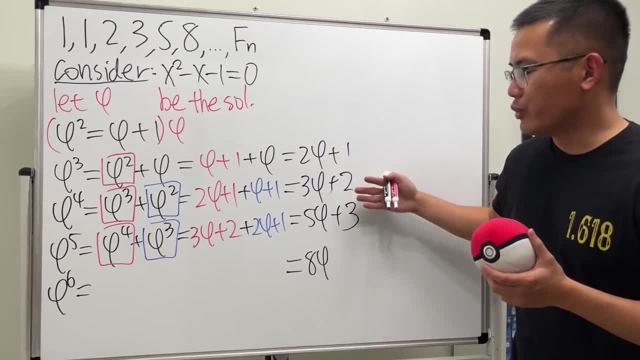 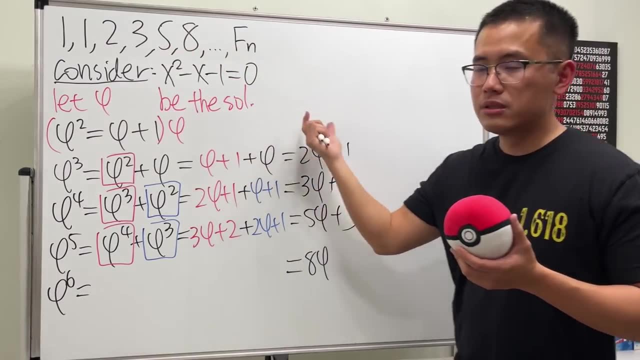 And of course it's valid, because the truth is, for phi 6, we're just adding the previous two expressions, And that's exactly how we get the Fibonacci sequence, Because for the next number we add the previous two numbers, Right? 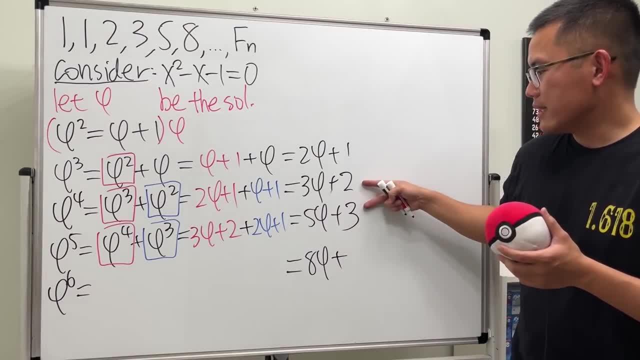 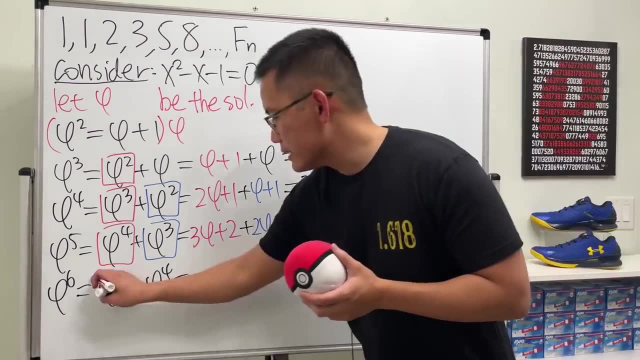 So, in fact, for the next one, we just add this and that together, which is 5.. And of course, if you want to show all the work phi to the sixth power, Same thing Told you. So of course, this right here will keep on going. 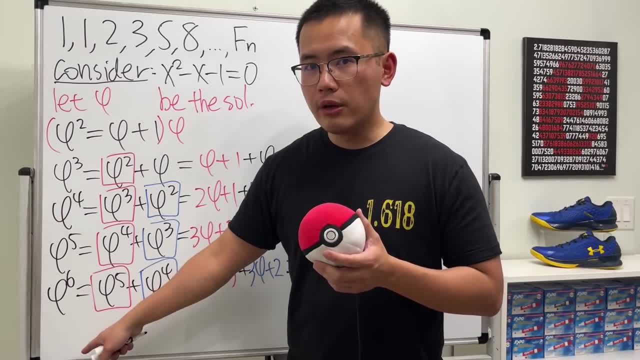 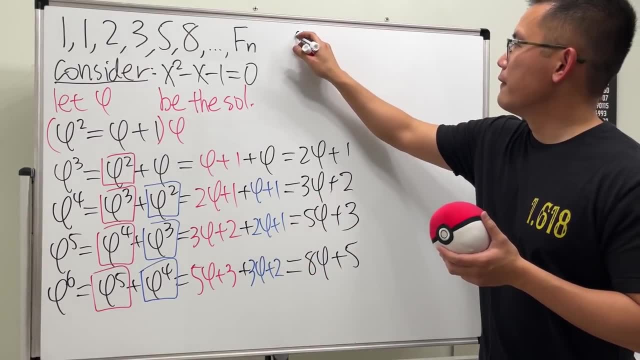 But now check this out. On the left-hand side we are talking about phi to a power n, So let's just go ahead and write that down. So notice, we have phi to the nth power. This right here will be equal to what? 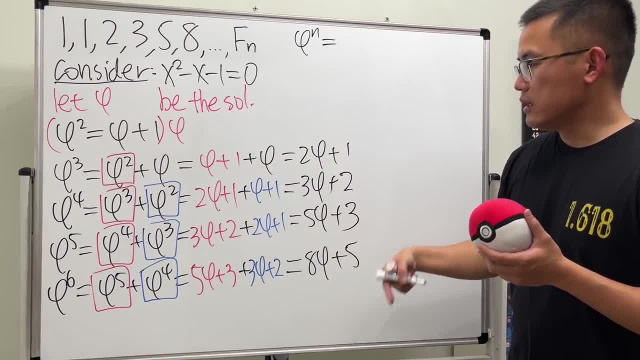 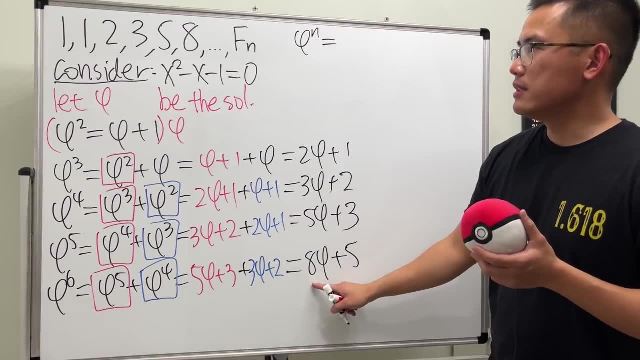 Well, the coefficient of phi right here is the Fibonacci sequence and that matches with the n Right, Because if you have, let's say, 6,, this is actually the sixth Fibonacci sequence: 1,, 2,, 3,, 4,, 5,, 6.. 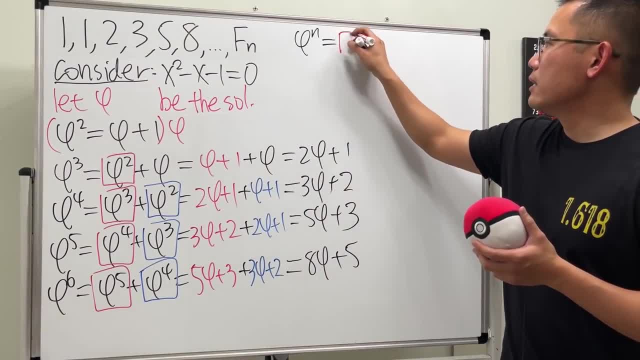 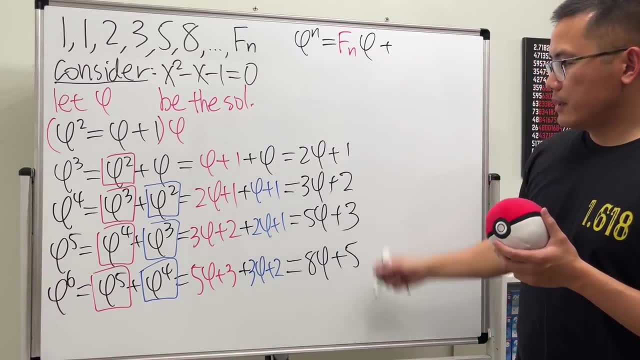 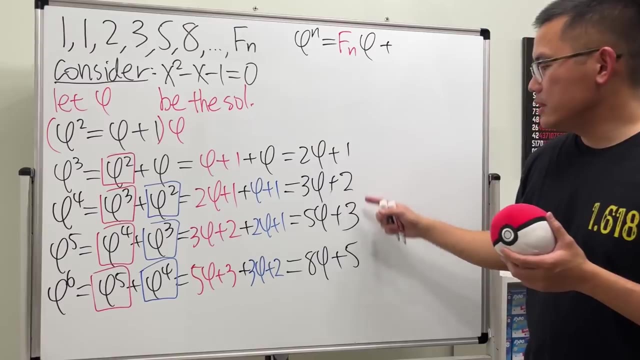 So this right here it will be Fn, And then we multiply by phi, which is the golden ratio, And then we add: How about the constant terms? Where do they come from? The truth is, they are also the Fibonacci sequence. 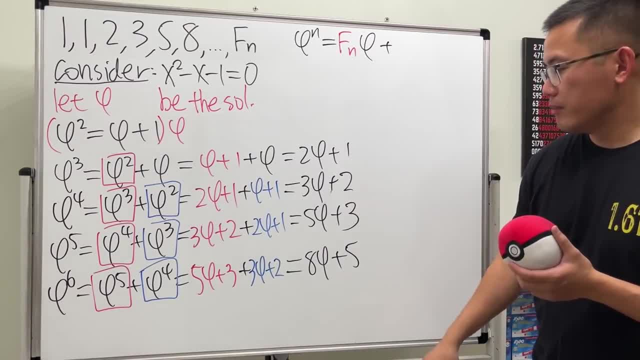 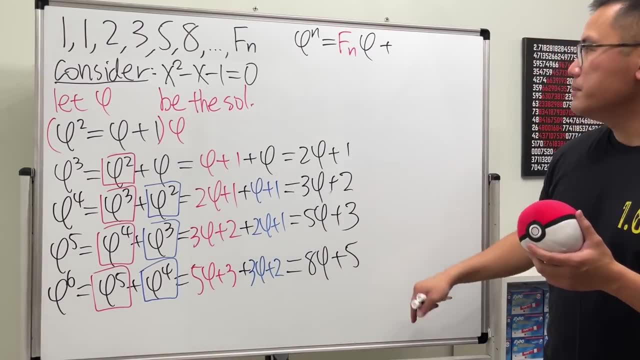 But the thing is that they are just the previous term. Right, The 5 is just the previous term. Right, The 5 is in front of the 8.. So for the constant terms it's just Fn-1, the previous term of the Fibonacci sequence. 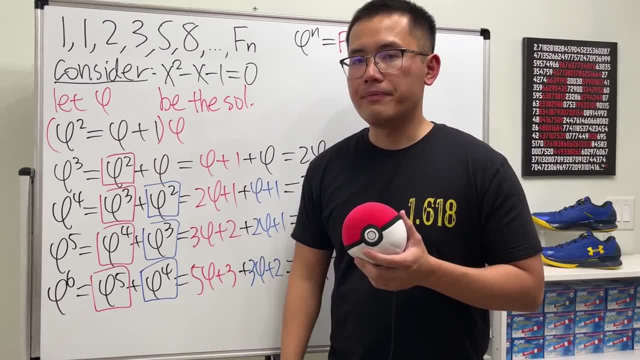 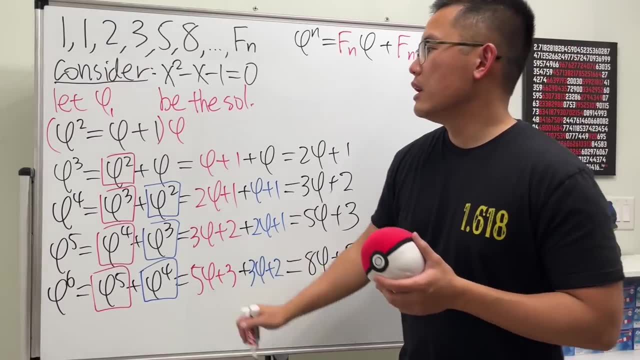 Cool. Now let's come back here again. Earlier we said: let phi be the solution, And technically we should say phi-1, because we have two solutions And the other solution I'm just going to call that to be phi-2.. 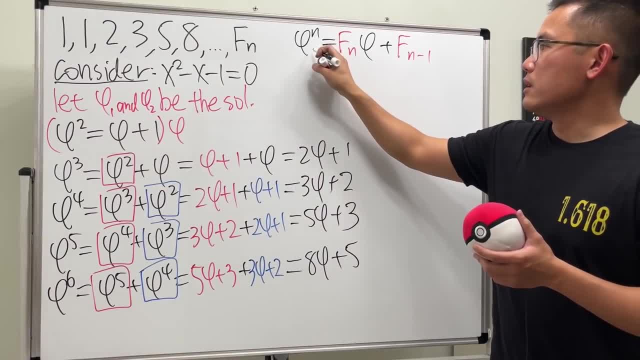 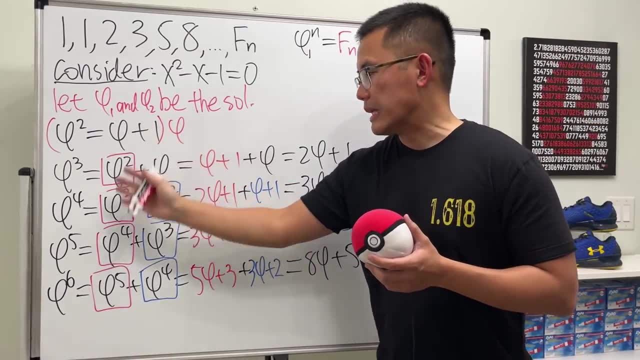 So earlier we were just dealing with phi-1, technically, So let me just put down phi-1 and phi-1 here, And because phi-2 is a solution as well, so the same thing will happen, Aha. 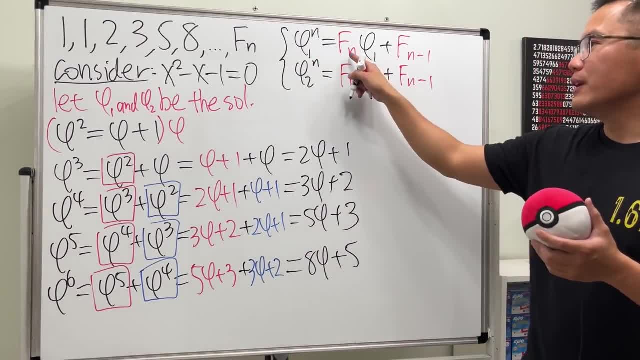 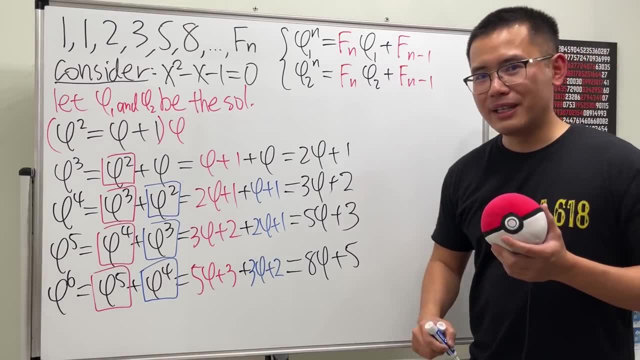 Now we have this kind of system equation to work with, And our goal is to find out what Fn is. Check this out. We have Fn-1.. We also have Fn-1.. Let's just go ahead and subtract these two equations. 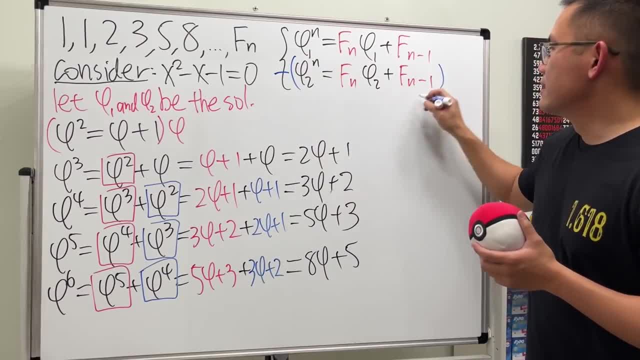 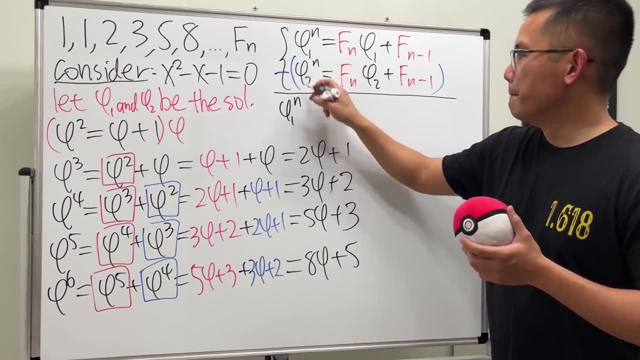 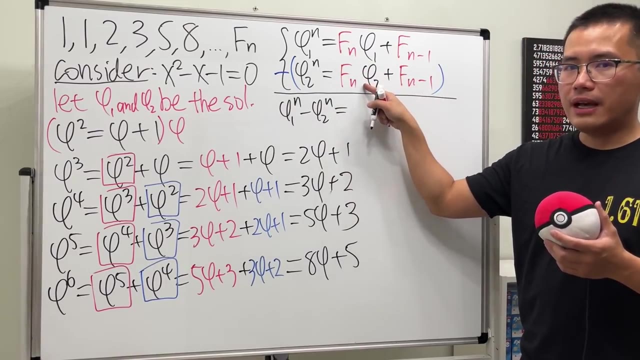 I'm just going to do the first one minus the second one, And then we will end up with: on the left-hand side, we have phi-1 to the n minus phi-2 to the n, And then on the right-hand side, okay, both of them have Fn, so we can factor that out. 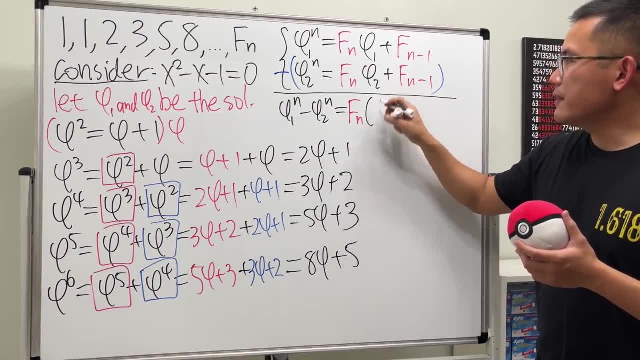 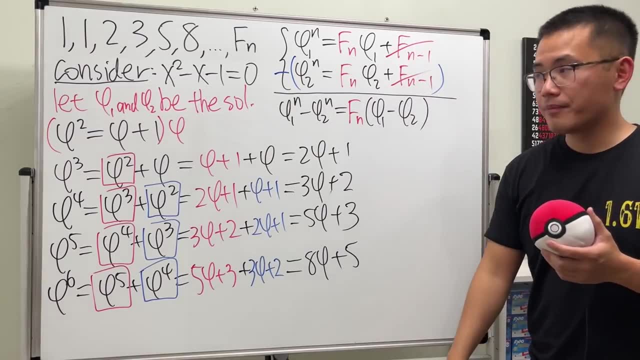 So I will just put down Fn, And then I will just have phi-1 minus phi-2. And then, of course, this minus that they cancel out. nicely Cool. So now let's actually figure out what phi-1 and phi-2 are. 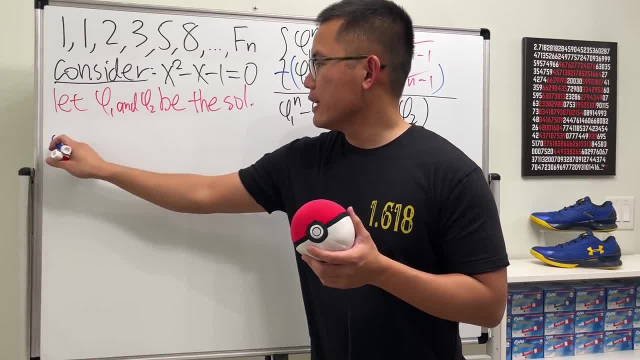 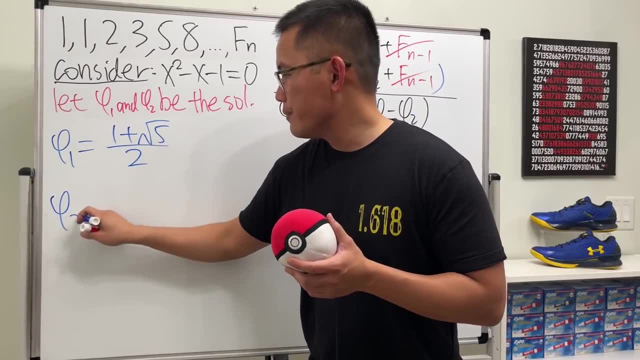 And of course we just have to solve this quadratic equation. And let's say: phi-1 is the golden ratio, which is 1 plus square root of 5 over 2.. And then for phi-2, well, this is just 1 minus square root of 5 over 2.. 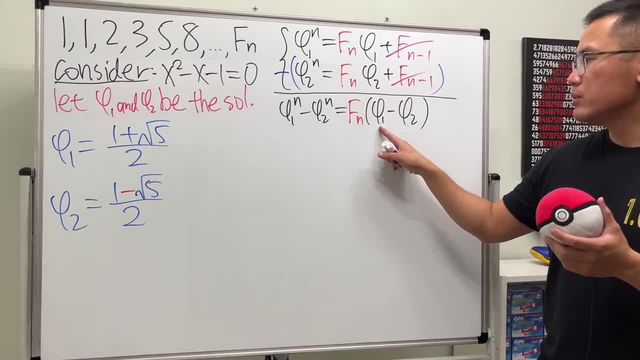 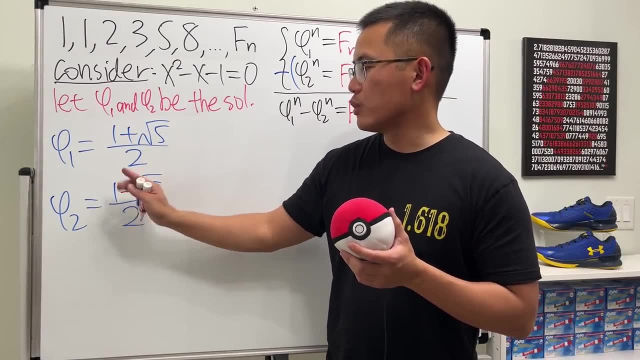 And right here we will have to get phi-1 minus phi-2.. This minus that they have the same denominator already. so we just do 1 minus 100.. Square root of 5 minus a negative square root of 5 is 2 square root of 5, but we have a 2 on the bottom. 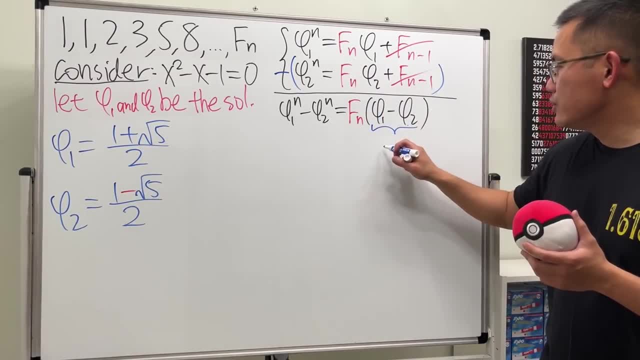 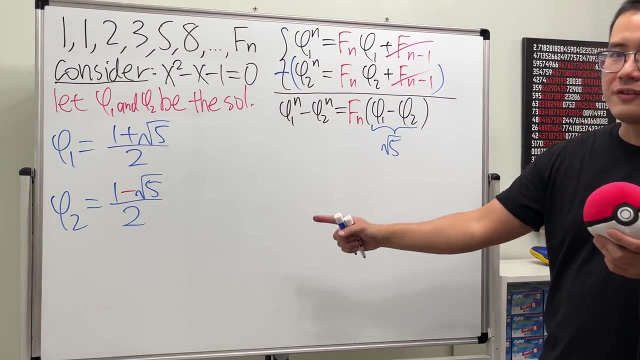 So, all in all this minus that, is just a square root of 5.. Now, ladies and gentlemen, to get this by itself, we just have to divide the square root of 5 on both sides. So Fn, this right here is just going to be 1.. 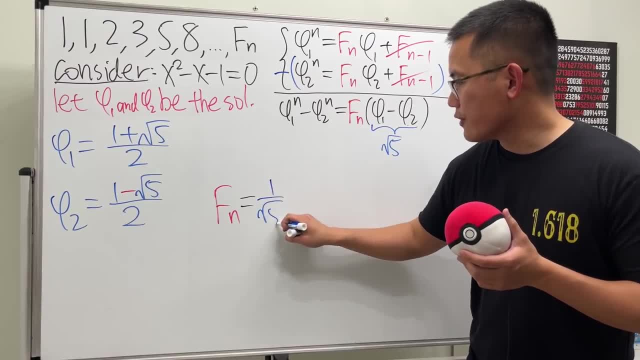 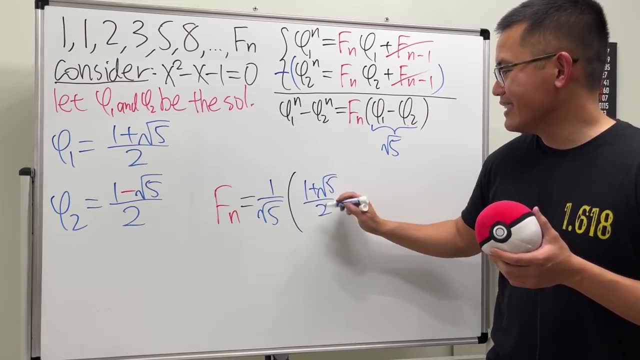 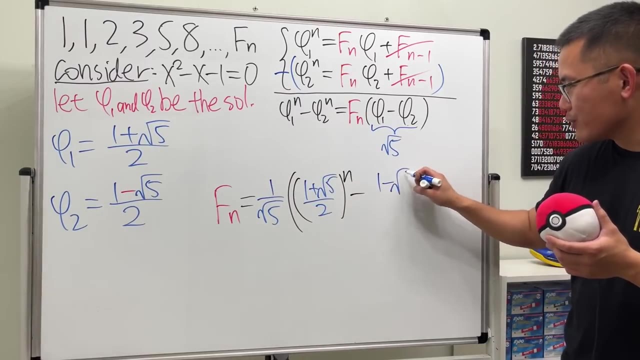 So Fn is going to be 1 over square root of 5 times phi-1. to the nth power, which is 1 plus square root of 5 over 2.. And then to the nth power And then minus phi-2, which is that 1 minus square root of 5 over 2.. 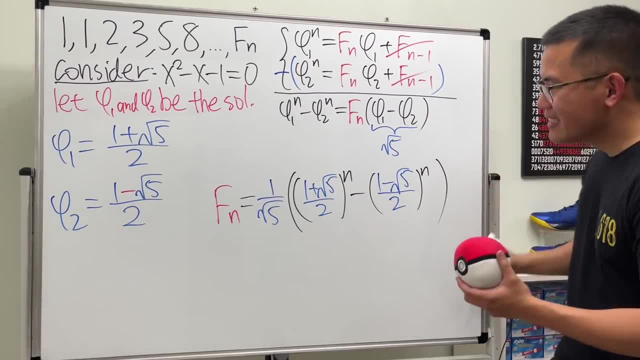 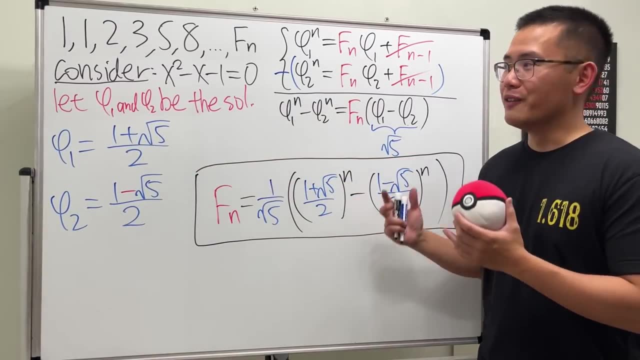 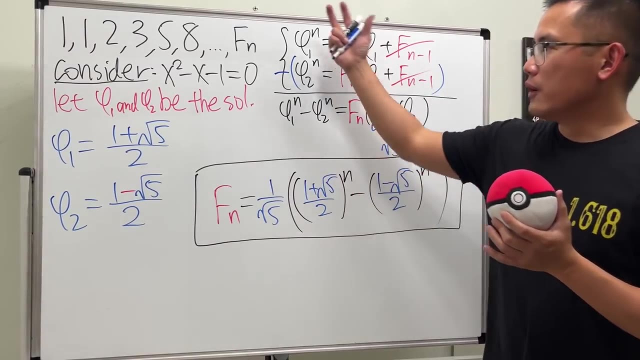 And then to the nth power, Ta-da. This right here is indeed the explicit formula for the nth term of the Fibonacci sequence. It's super, super cool, Because usually I will show you guys how to solve the formula by using the difference equation. 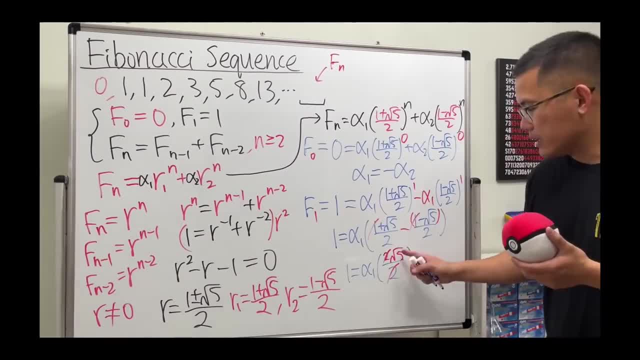 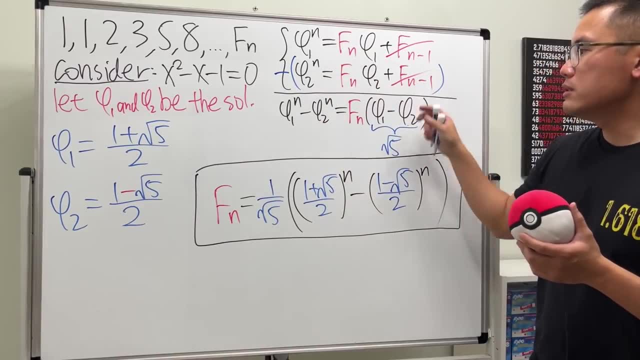 but that's a little bit technical, because you might have to take a discrete map in order to encounter that situation. But for this we saw the pattern earlier and then we're able to come up with this, and then it works out. so so, so nicely. 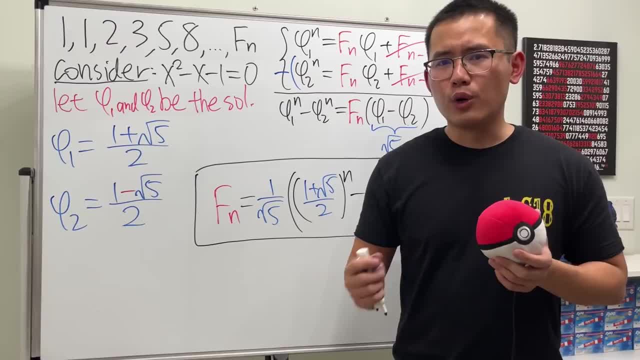 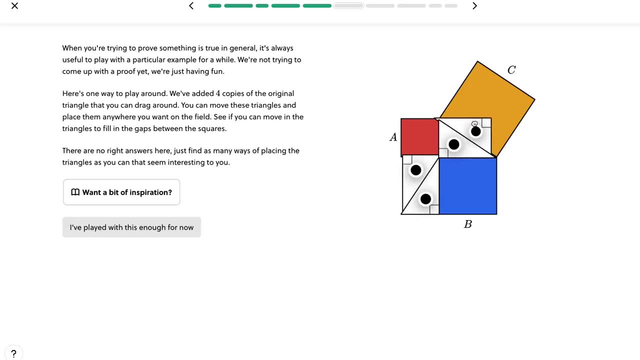 And if you guys like math, I'm pretty sure you guys will also like today's sponsor, Brilliant. As a calculus teacher, I'm always looking for new resources to help students learn better, and at Brilliant they provide exactly just that. The best thing is that they focus on interactive learning. 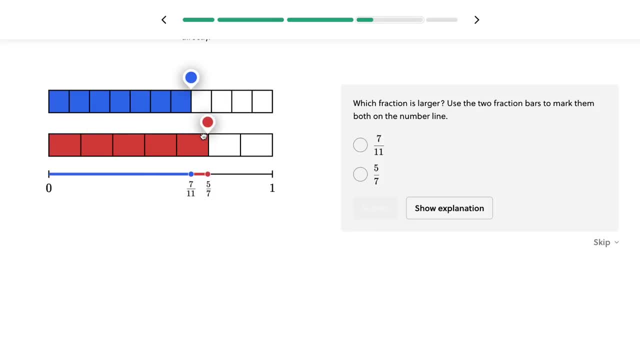 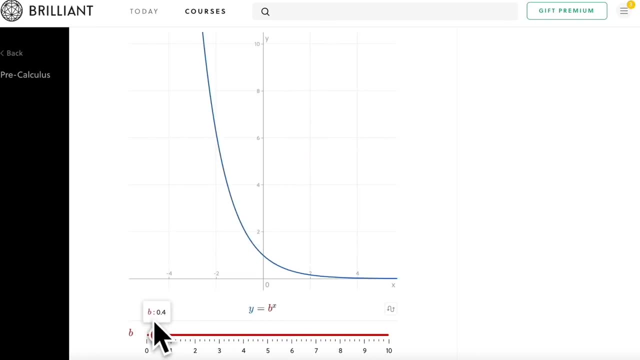 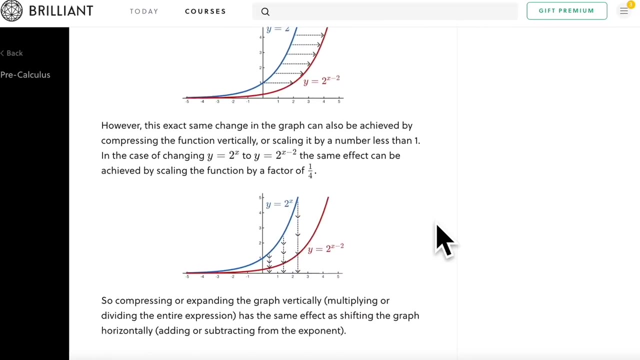 and all of their courses in math science and computer science are all based on that fundamental. One thing I really enjoy is that they provide interactive lessons so that you can easily see how the function is changed when the number is adjusted. I really like them because they also believe that the best way to learn is by actually doing it.